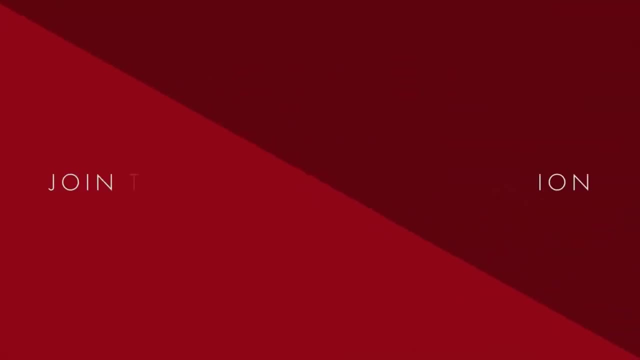 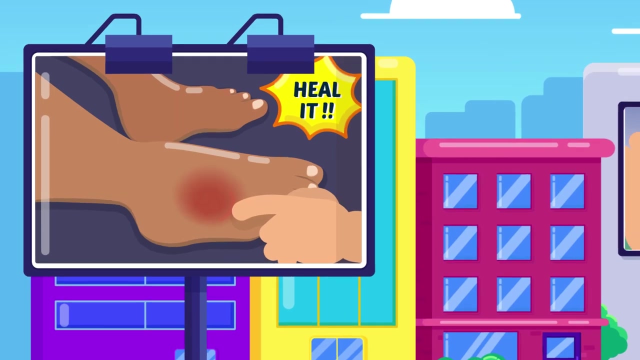 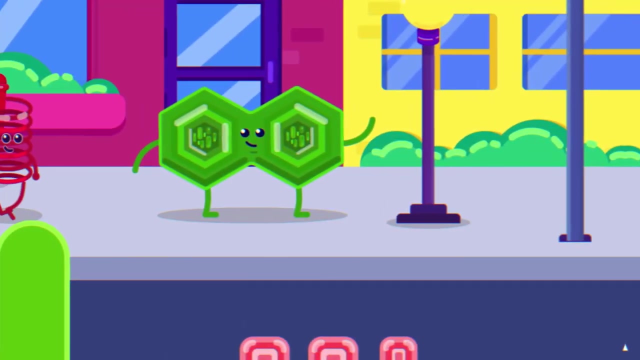 Vitamins Deficiency. diseases such as scurvy and beriberi are caused by the lack of certain chemical substances in our diet known as vitamins. Vitamins are organic compounds that are not built in a definite pattern like carbohydrates, proteins and fats. They are not energy-providing. 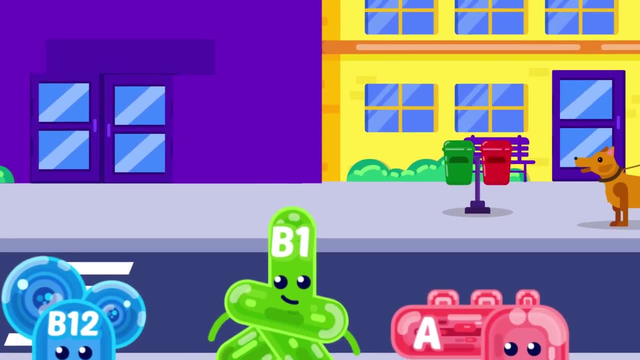 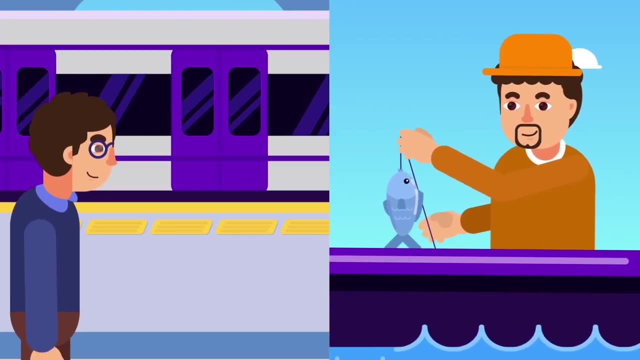 foods nor bodybuilding foods. Yet they are required in small quantities by animals, including humans, for normal health and development. In both underdeveloped countries and developed countries a deficiency of vitamins can arise. How you ask In developed countries people? 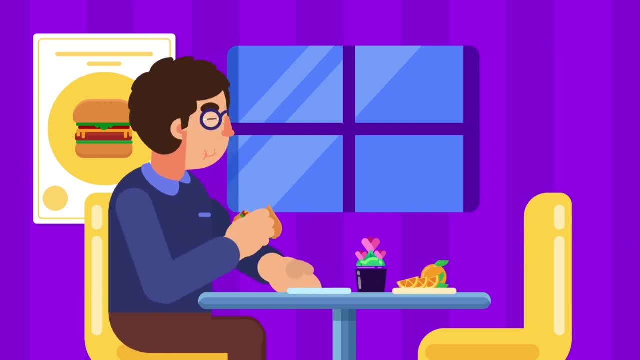 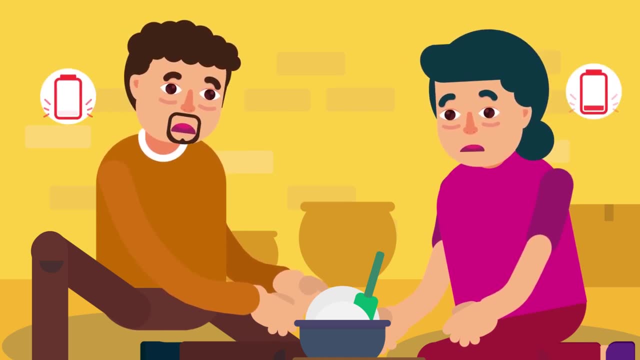 eat processed foods more, and thus vitamin-rich raw fruits and vegetables are avoided. In underdeveloped countries, people do not get a balanced diet and so are malnourished, resulting in vitamin deficiency. Vitamins can be grouped into two types: fat-soluble and water-soluble. 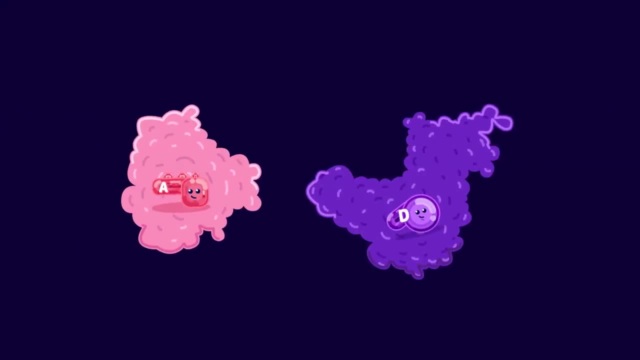 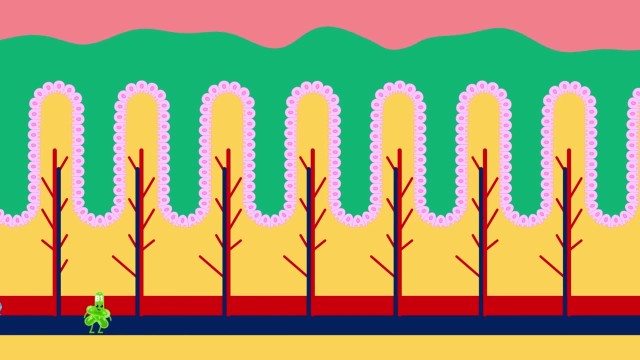 Fat-soluble vitamins. Vitamins, as the name suggests, are soluble in fats and can be stored in the fats of the body. But water-soluble vitamins cannot be stored in the body and need to be supplied in the daily diet. When a particular vitamin is deficient, characteristic symptoms appear. 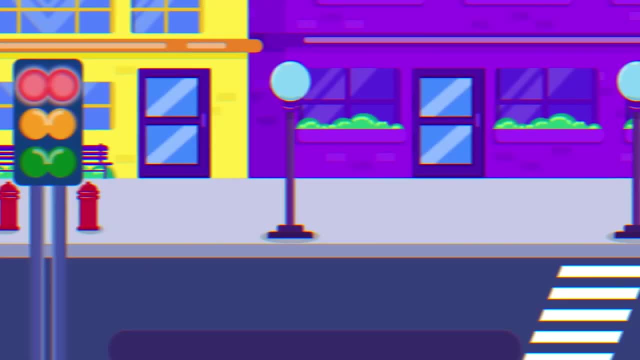 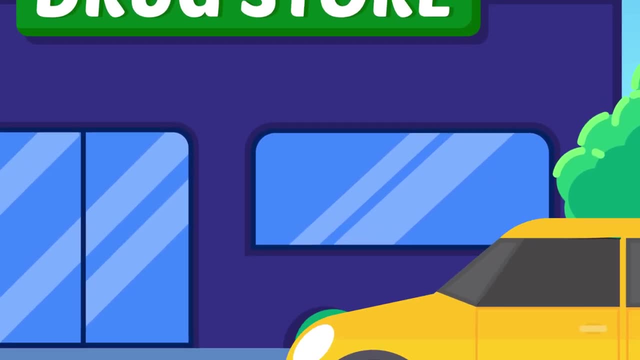 Usually a mild vitamin deficiency is hard to detect, but it may impair a person's well-being so he feels run down or irritable. If the deficiency is severe, the particular deficiency disease will develop As vitamin supplements are becoming easily available over the counter. 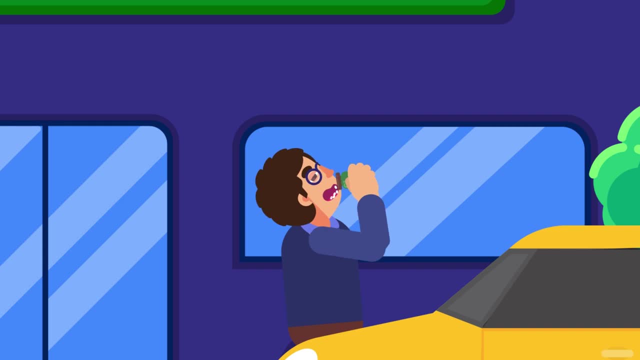 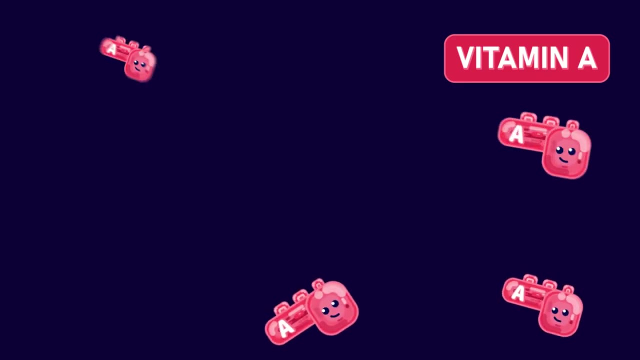 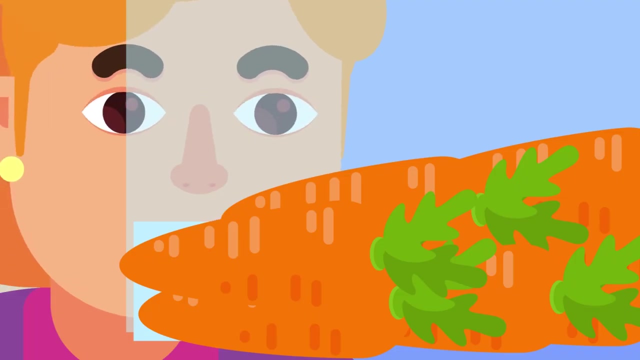 we must take precaution of the dosage while consuming them. Larger quantities of some vitamins are toxic and may produce mild diseases, and should only be taken when prescribed. Source and functions of vitamins. Vitamin A: Ever heard carrots are good for our eyes. How is that? 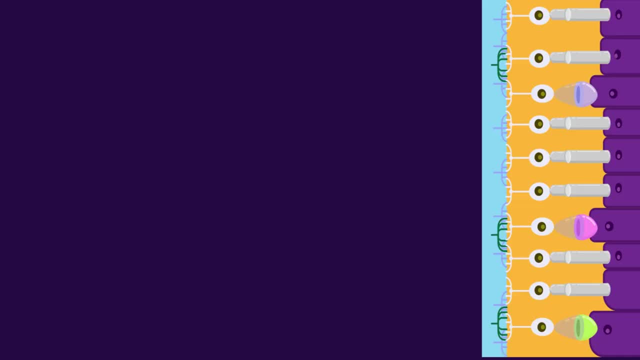 Carrots are a rich source of vitamin A, a fat-soluble vitamin, and is required for the formation of a light-sensitive pigment in the retina and for maintaining healthy epithelial tissues. Rich sources of these vitamins include vitamin C, vitamin C-1, vitamin C-2, vitamin 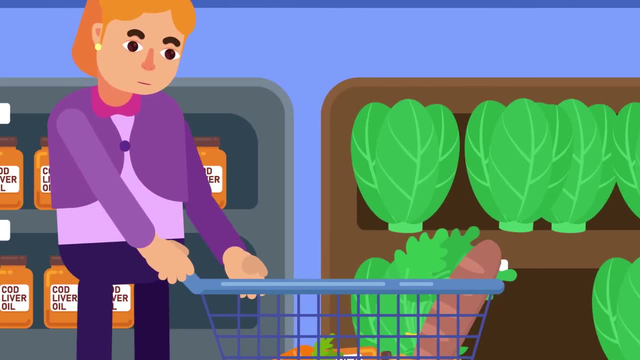 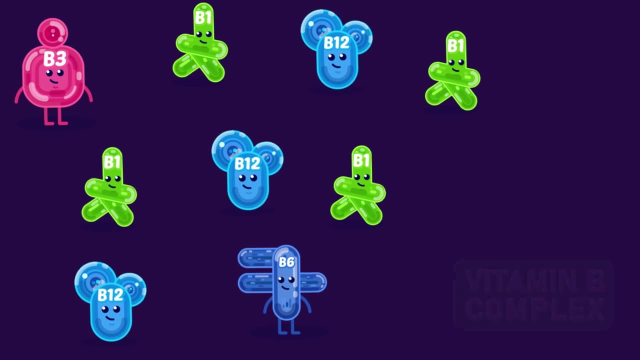 C-3,, vitamin C-4,, vitamin C-6, and vitamin C-7.. Rich sources of these vitamins include dairy products, fish liver oils and green leafy vegetables. Vitamin B complex. Vitamin B has many subtypes, many of which are important coenzymes in cellular respiration.